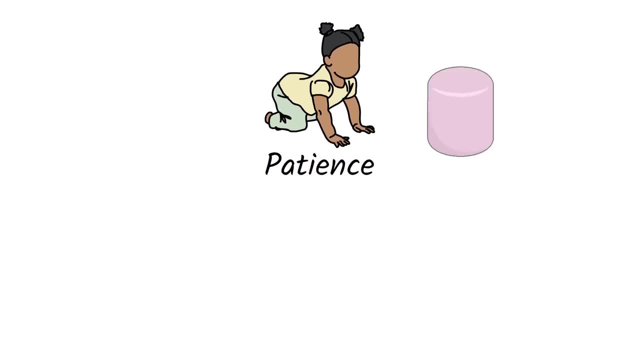 2. There is a famous experiment called the marshmallow test, where young children were given a marshmallow and told that if they didn't eat it right away, they'll get a second marshmallow. What is interesting is that researchers followed this group of kids for decades and found that those 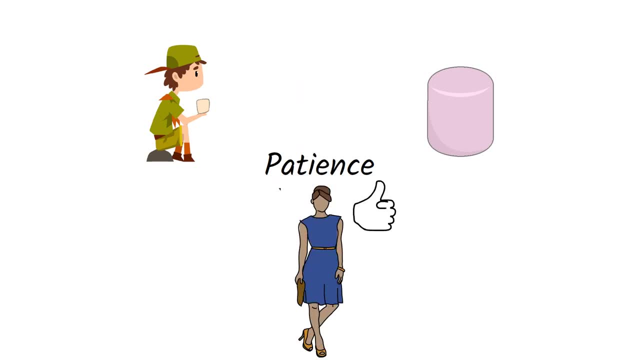 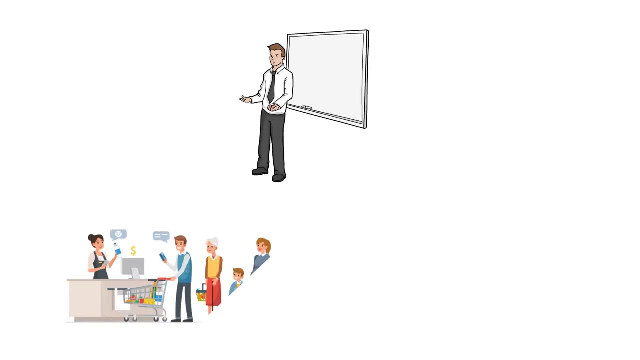 kids who waited for a second marshmallow ended up significantly more successful as adults. They had better relationships, achieved higher levels of education and earned more money on average. The great news is that patience and delayed gratification can be taught, And this can be done in many ways: at the checkout line in the grocery store or the 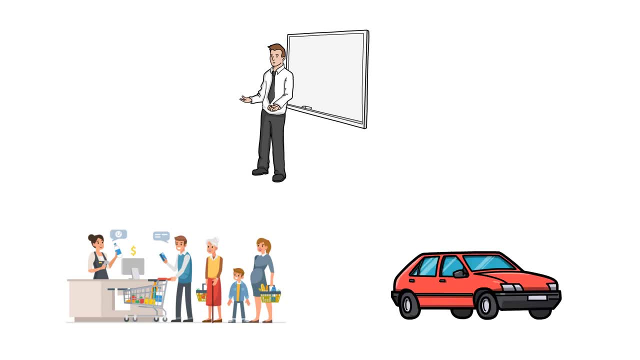 car ride on the way to the park. A great method to use is to remind them that there's a light at the end of the tunnel and they can get what they want if they are patient and show them fun ways to distract themselves. to make time go faster. This can be a great age to begin saving money together. 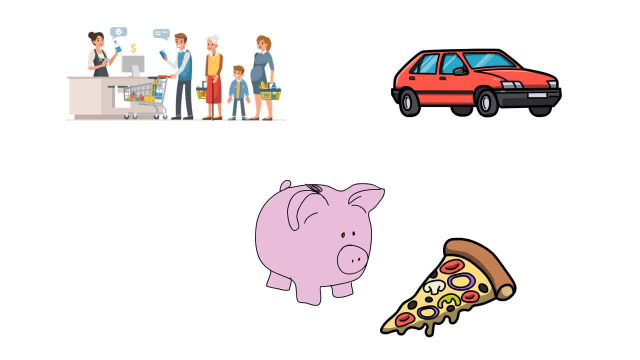 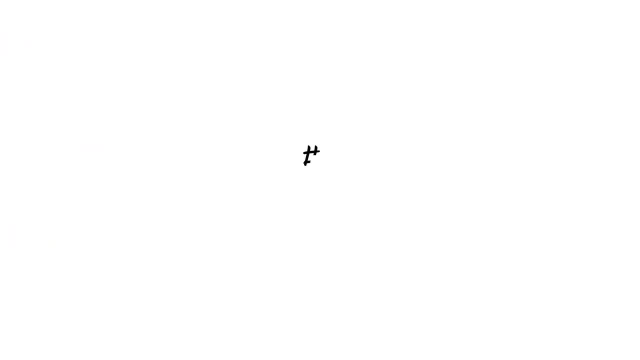 whether it's for a specific reason like buying a pizza or a trip to the water park, It can be a great practice to teach the importance of saving money by actually doing it together. 3. There are many ways to save money. Number 2.: 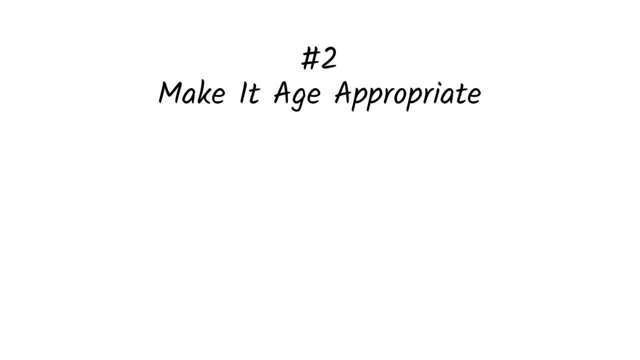 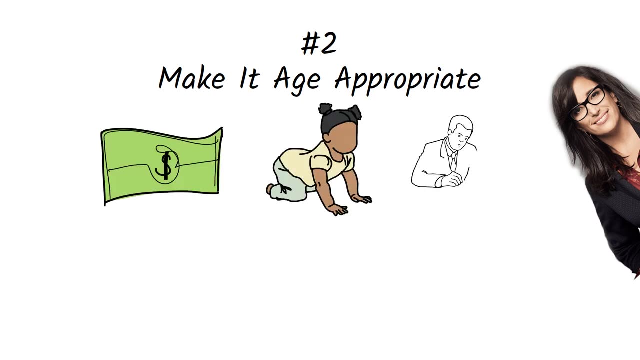 Number 2.. 2. Make it age appropriate. According to Kobliner, it is important to adapt the message to the kid's age level, Teaching kids of preschool age that money has value, where money comes from, that money can be exchanged for things and begin creating. 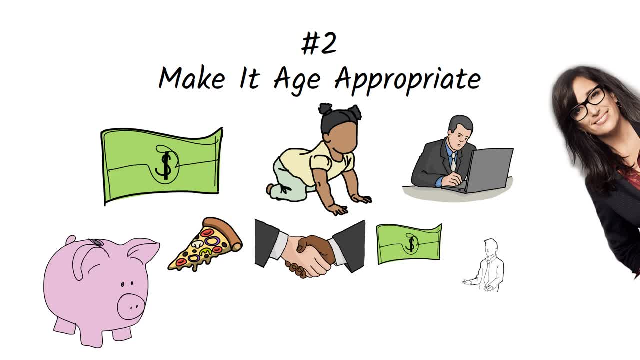 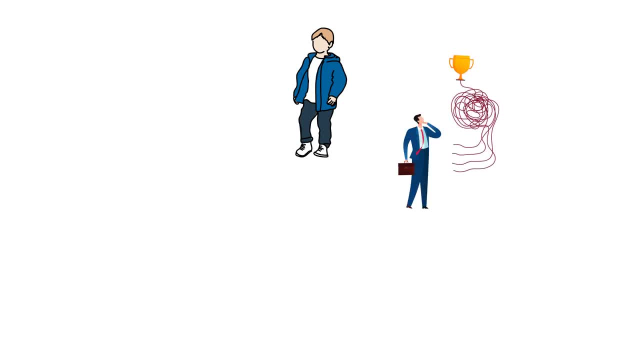 a habit of saving can be a simple yet a great way to start a foundation of good money habits For an elementary schooler, teaching a concept of opportunity, cost and how sometimes they have to stop spending money on the daily Doritos bag to be able to save money to pay for the 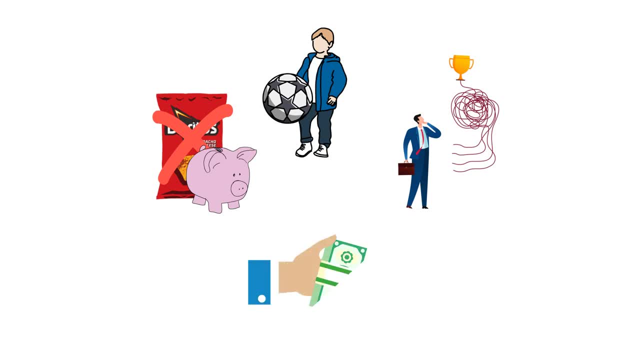 toy they want. This is where kids begin getting fascinated with earning money so they can do odd jobs or extra jobs in the house outside of chores. This can also be a great age to teach the concept of interest and how some banks keep your money safe while giving you. 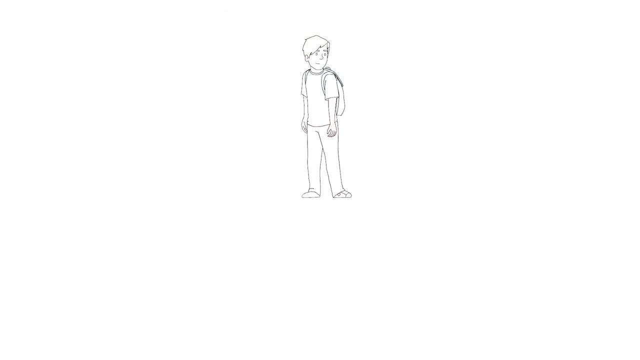 a small percentage of free money. In middle school it can be a good idea to teach the importance of always having money around, or, as Kobliner says, it is never good to have no money. It is fine for a kid to save money to buy an item, but focus on not. 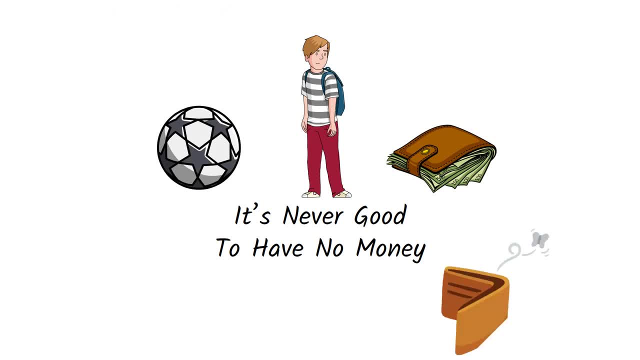 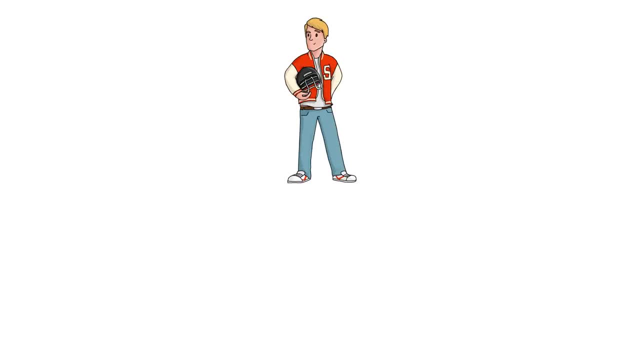 spending every penny we have on it. If a purchase wipes out their entire bank account, then it's a good idea to wait and save a little more before buying. In high school is where we can begin earning money and saving for important parts of their 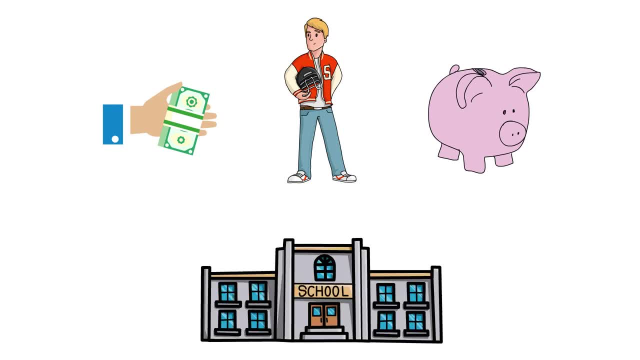 life, such as college. Research shows that kids whose parents carry the full burden of college cost score lower GPAs than kids who chip in. Although the reason is not clear, the most accepted theory is that when a kid feels he or she has some skin in the game. 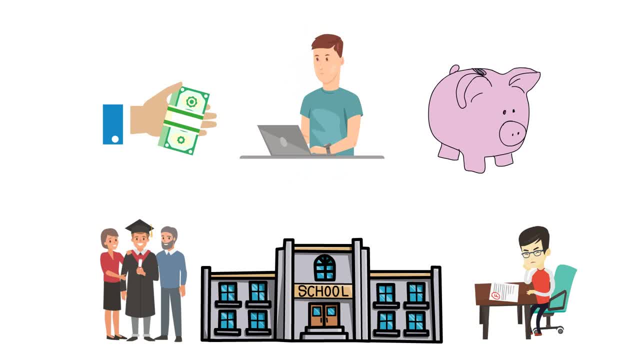 they will be more motivated to take full advantage of the money they have saved. When they lose a $20,000, they will go through a lot of extra work and tears. So, with all that said, what will we mean to them if they take full advantage of this sacrifice? 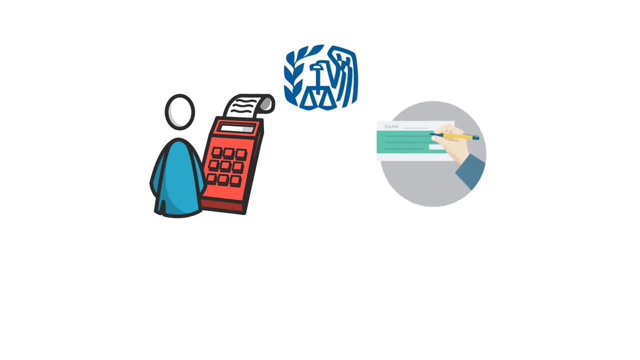 This is also a great time to teach kids about the reality of taxes. Usually, this is where kids first begin getting jobs and receiving paychecks, so this is prime time to teach why their tax will be smaller than expected. This is where we can teach about the deductions. 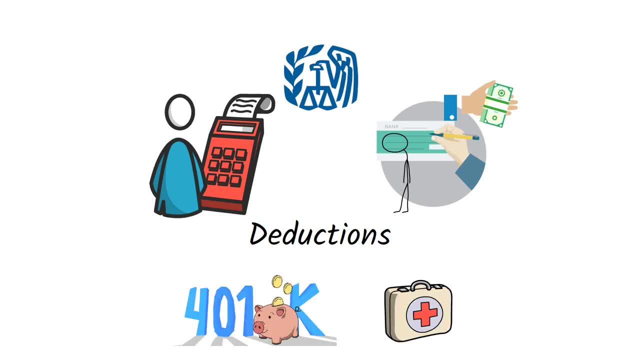 that can be used before the government takes taxes out, like 401k contributions, health insurance or any flexible spending account. It can be a good idea to contribute to a 401k willing to match, since this is essentially free money. We can also teach that there are generally 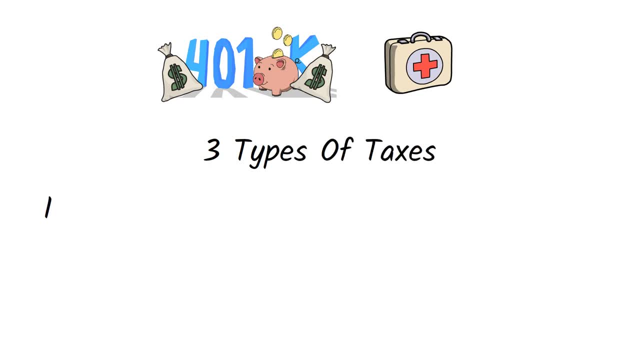 three types of taxes that get deducted from their paycheck: Income tax, which is federal, state and sometimes local, which helps the government fund schools, highways and more. They'll also pay social security and medicare taxes. It is important for them to understand the difference. 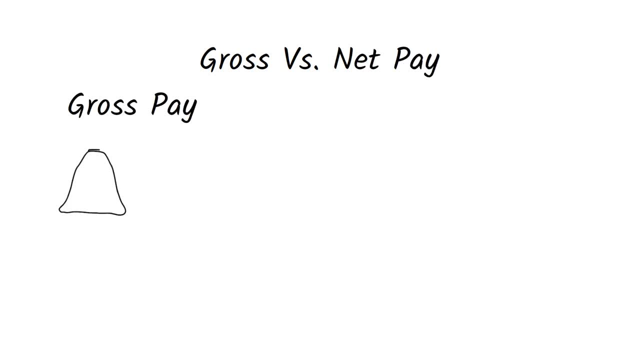 between gross versus net pay. Gross pay is the amount you earn before taxes are taken out. Net pay is the amount you receive after taxes and other deductions are subtracted. This is where we can talk about investing, compounding interest and the benefits of. 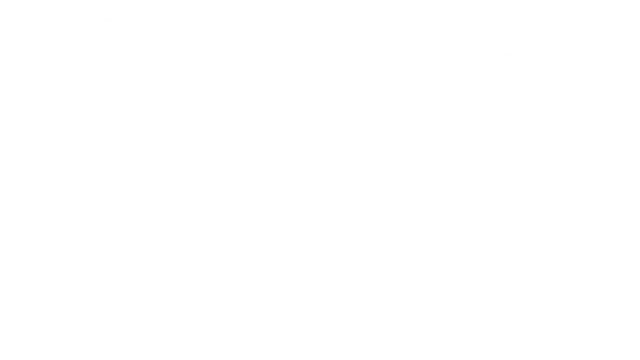 building an investments fund. Using an example like: if he invests $500 into an investments account like a Roth IRA or an index fund at the age of 16, with an 8% growth rate, by the age he's 65, these $500 will turn into over $20,000.. Keeping these topics age-appropriate can help. 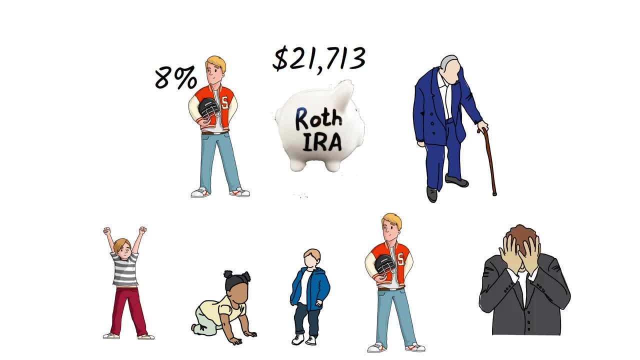 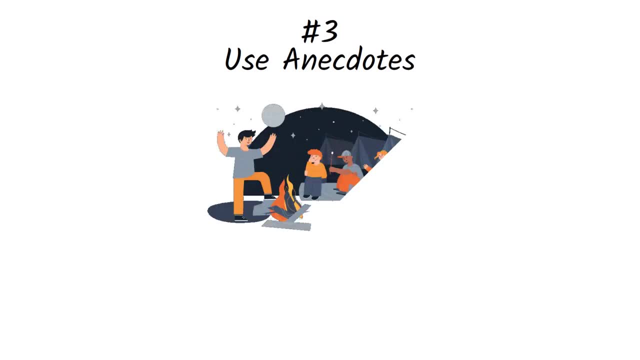 the kid enjoy learning and learning more about the world. Number 3. Use anecdotes. Most people, not just kids, learn better when we use stories to convey a message, And it is no different with money. Many parents understand that when they go into 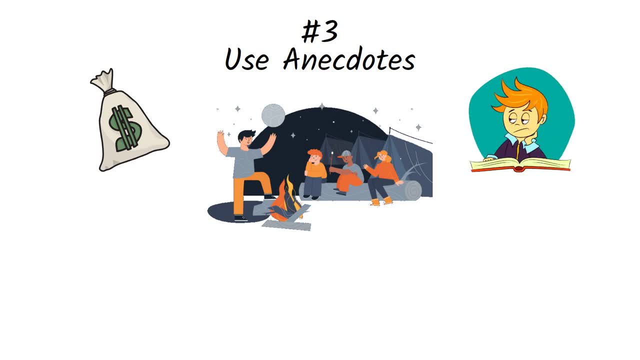 lecture mode, their kids tend to tune out or, worse, they actually do the opposite of what was told. If you tell your high school kid how a friend couldn't get an apartment to live in because she ranked a lot of credit card debt from overly shopping the year before, will create a 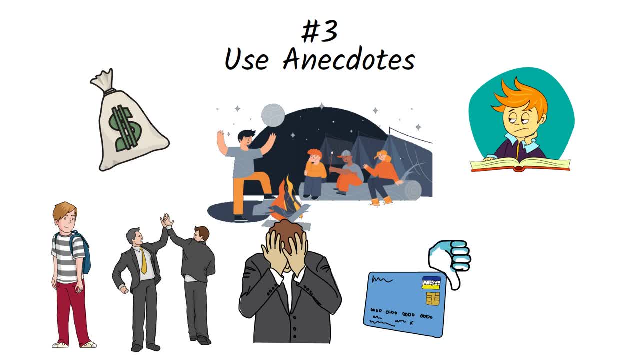 longer period of time for the kid to learn about money And if you tell your high school kid how a friend couldn't get an apartment to live in because she ranked a lot of credit card debt from overly shopping the year before will create a longer period of time for the kid to learn about. 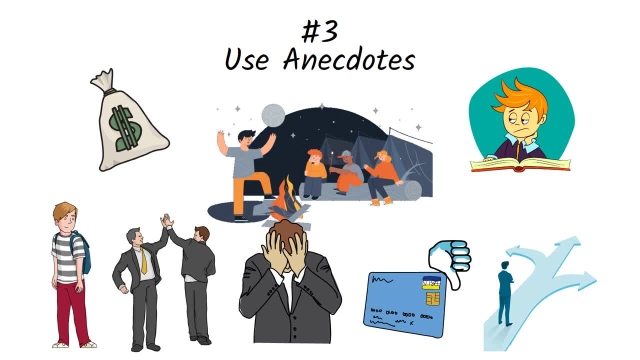 money. I'm glad each of you have in-depth knowledge about your son's future and reaches higher levels of maturity and results than anyone else's education. anybody knows and will soon live. you see every detail that we know. Now let's add more statistics to let you know. 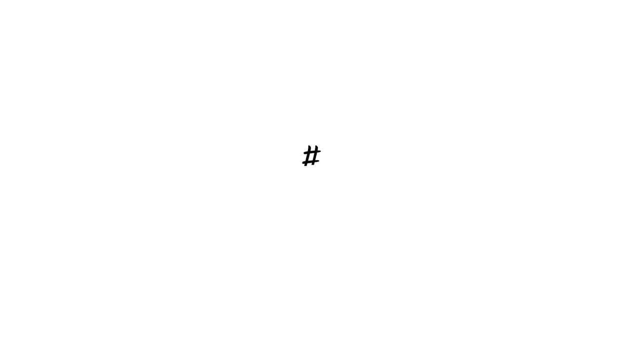 We generally remember that too many people tend to show a story that can win over a child's passion for education, but never, no one can turning a blind eye to that story without engaging anyone's attention. So this is a dynamic way of awestrucking people that want to. 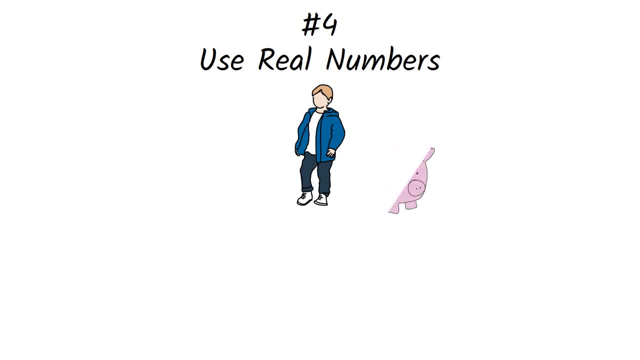 learn. We often come across stories that areまだ few ways to� apply a stunning idea to what to think of children and what to do about it, but that them that if they invest $300 a month in a retirement account, starting at the age of. 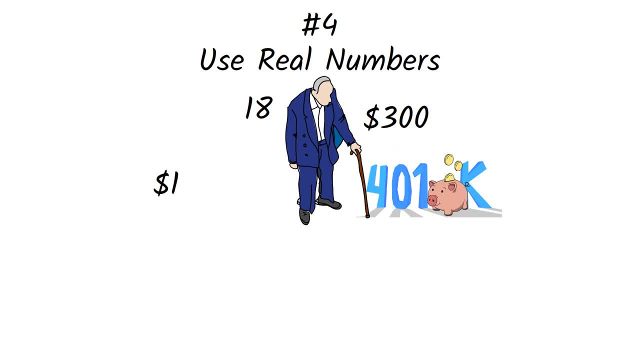 18,. by the time they are 65, they will have over $1 million. The word $1 million inevitably makes the high schooler take notice and have a stronger impression of the importance of saving for retirement. If you're not sure where to get your numbers, there's a great free tool that will help. 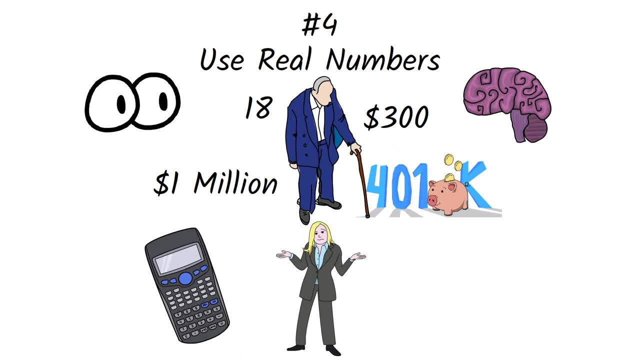 you calculate the compounding interest based on interest rates, amount saved and length of time. This is a government site called investorsgov And no, this is not sponsored. just really like the tool to calculate the compounding interest of any investment. 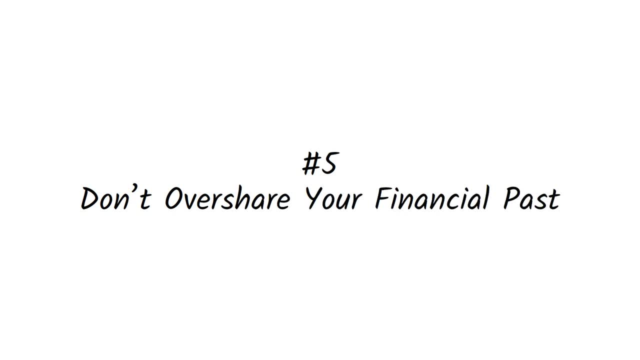 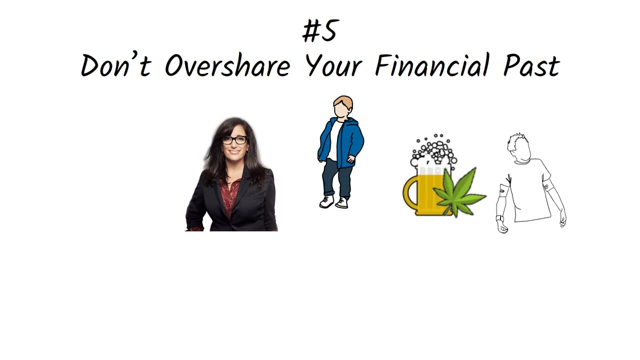 Number 5. Don't overshare your financial past. There's been studies that show that kids whose parents share details about their past indulgence in drugs or alcohol are more likely to also indulge in those behaviors In a similar way. Kobliner suggests that telling your kids about the time you empty your bank. 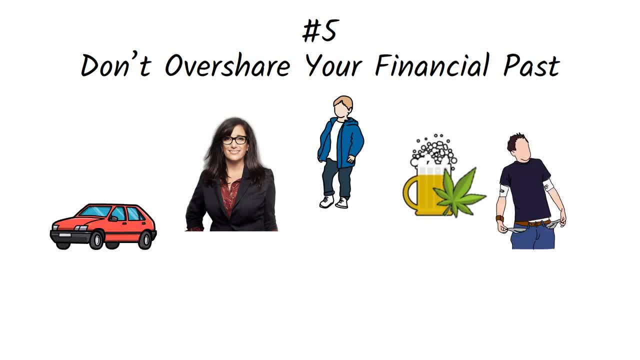 account. to go on a road trip with your girlfriend might actually glamorize this behavior, even if you tried to tell them it was a bad idea. Most of us had made bad financial decisions at some point in our lives, but there's no need for your kids to know that. 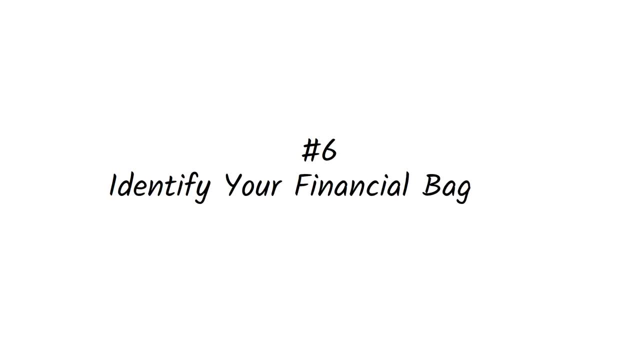 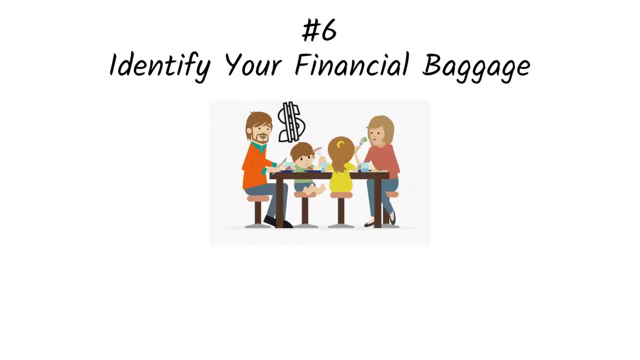 Number 6. Identify your financial baggage. then leave it behind. For many people, their parents never taught them about money or got their money habits as a result of their parents' behavior, Whether they copy their parents' financial patterns or do exactly the opposite there. 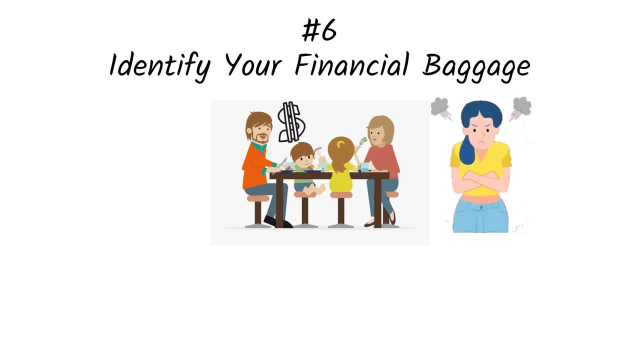 are many people who blame their financial habits on their parents. So what do you do? Ask your parents. Although it's always a good idea to be aware of how your parents handled money and how that has affected your financial behavior, it's not a good idea to use it as an excuse. 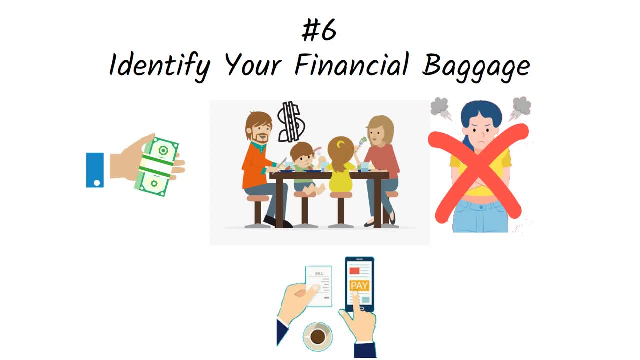 to explain away your bad money habits or, worse, avoid teaching your kids about money. As Kobliner says, identify your financial baggage, then leave it behind. Approach money in a positive way, even if it's not easy at the beginning to avoid. 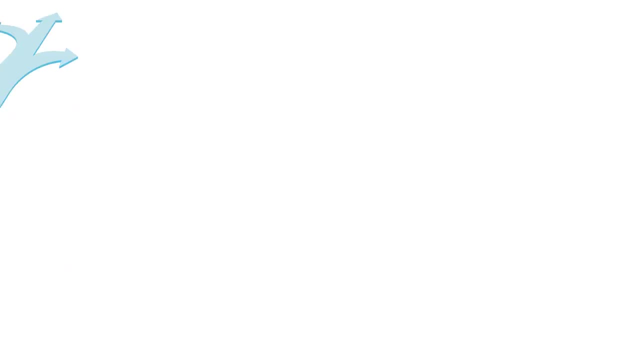 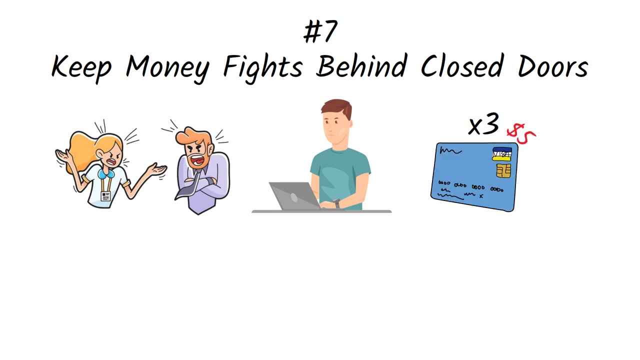 passing this negative feeling about money to your kids. Number 7. Make money fights behind closed doors. Researchers have found that college students whose parents regularly fought about money when they were younger were three times more likely to have credit card debt of at least $500 or more than kids whose parents kept their financial peace. 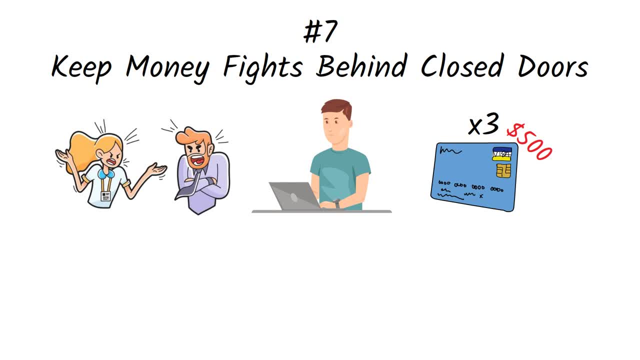 It is very likely that you and your partner might not agree on every money decision, but it is important to shield kids from big money disagreements. A good idea is to create a money timeout for parents only to discuss money decisions, and if it's related to money, then it's a good idea to create a timeout. 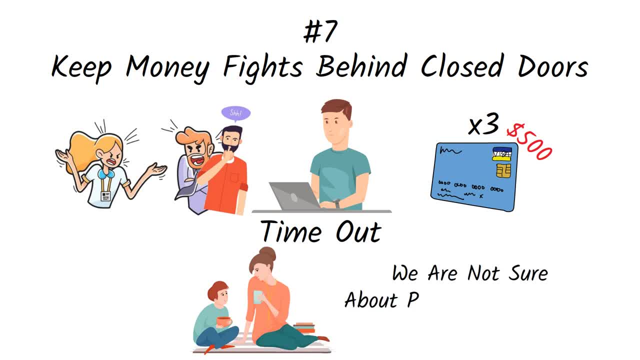 If it's related to the kids, for example, you can simply tell them we're not sure about paying for that yet. we'll discuss it and get back to you. This can show them that you take the time to make those decisions logically instead. 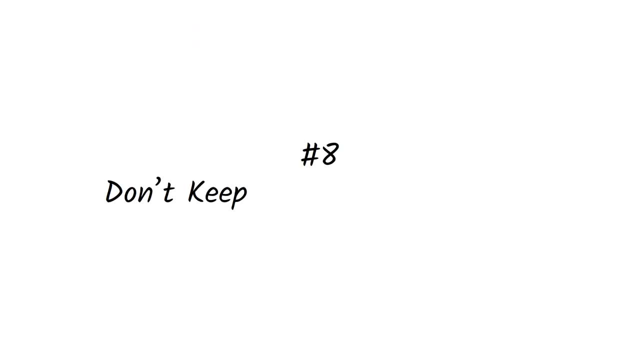 of, emotionally, Number 8.. Don't try to keep up with the Joneses or the Kardashians. It is natural to make comparisons with other people, and living on a consumer-centric, media-driven culture doesn't help. Nevertheless, it is important to fight the urge to compare your family's money choices. 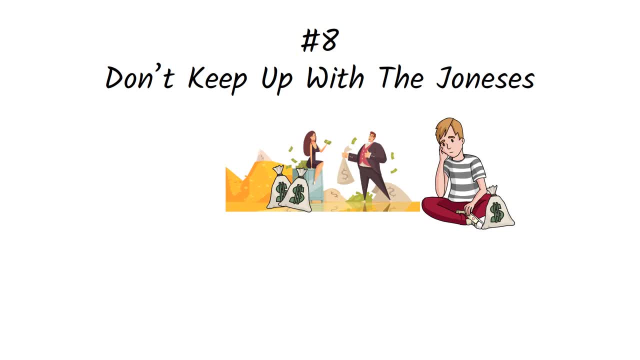 with anyone else's, Especially within the hearing-blind community, It is important to make comparisons with other people's money choices. and it is important to make comparisons with other people's money choices. Research shows that comparing aspects of their financial life with others make people generally. 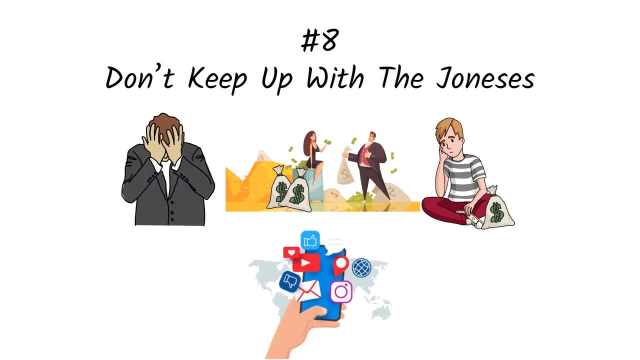 less happy, especially in the world of social media, where we can easily see those with better, or who appear to have a better, financial life. This can be a particularly dangerous trap If you want to teach your kids to avoid the trap of keeping up or looking down on their